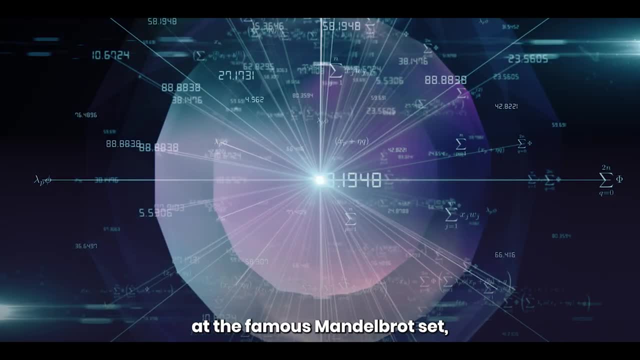 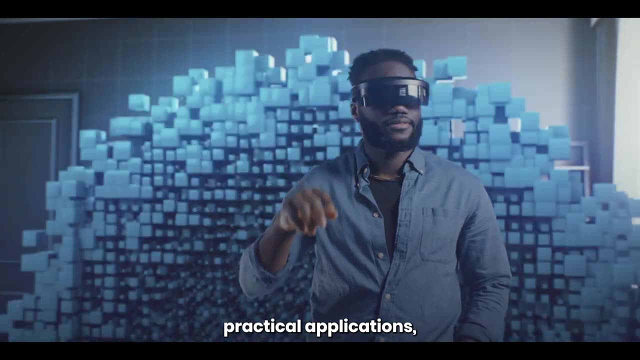 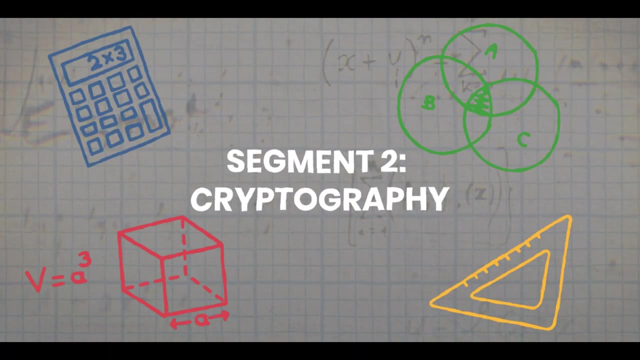 scales. Let's take a look at the famous Mandelbrot set, a fractal that exhibits infinite complexity and beauty. Fractal geometry has numerous practical applications, such as in image compression, computer graphics and even the design of antennas Cryptography. 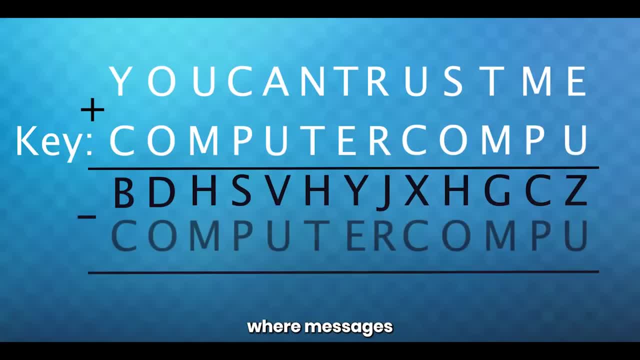 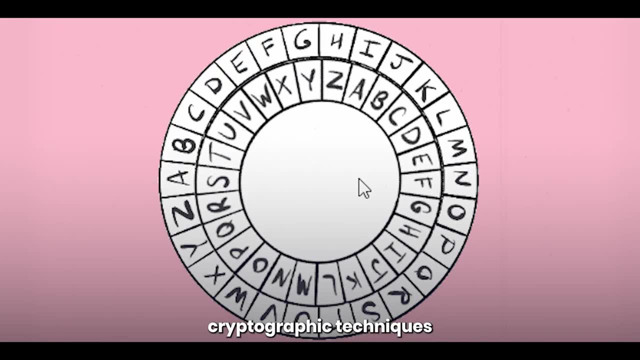 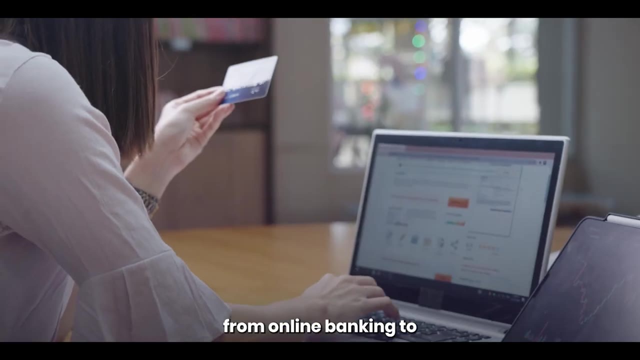 Cryptography is the science of secure communication, where messages are transformed into a code that is difficult to decipher without the key. One of the earliest and simplest cryptographic techniques is the Caesar cipher. Cryptography has a vital role in modern communication, from online banking to military communication. Without cryptography, our sensitive information. 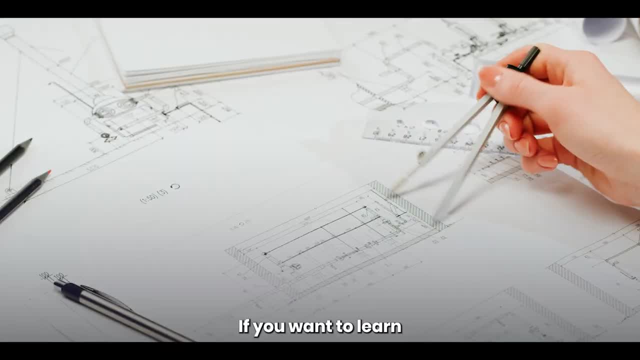 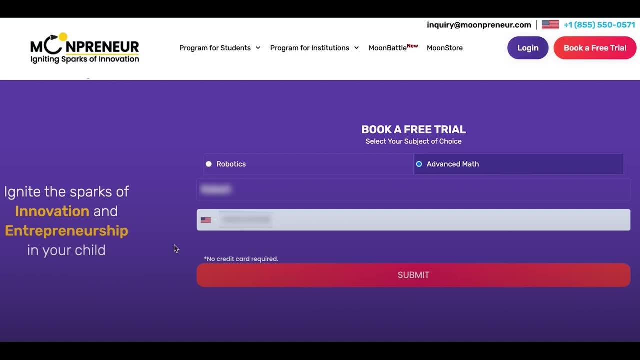 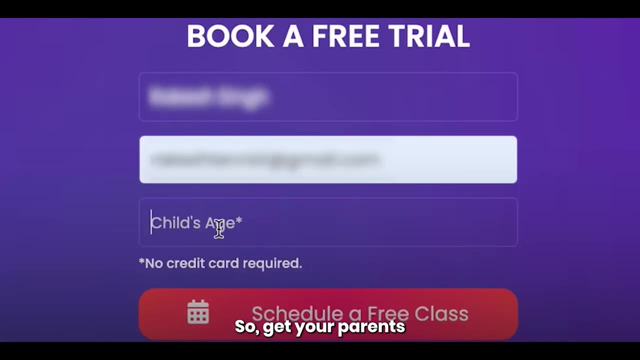 would be vulnerable to theft and interception. If you want to learn more about math projects, Monpreneur is offering a free advanced math class for grades 3 to 6.. But you've got to hurry, Because this offer won't last forever, So get your parents to sign. 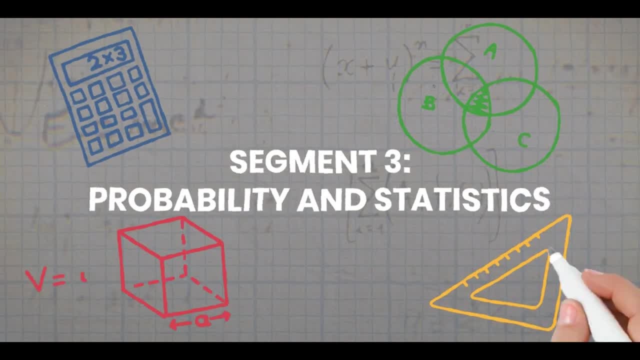 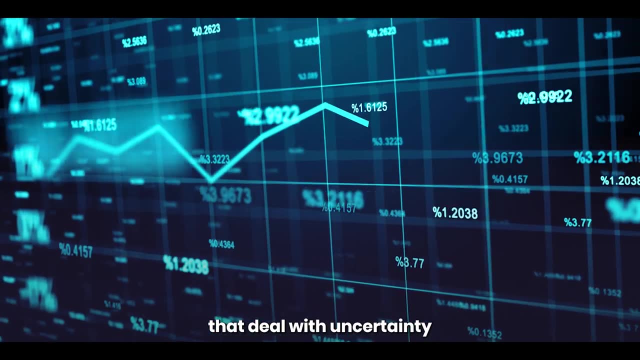 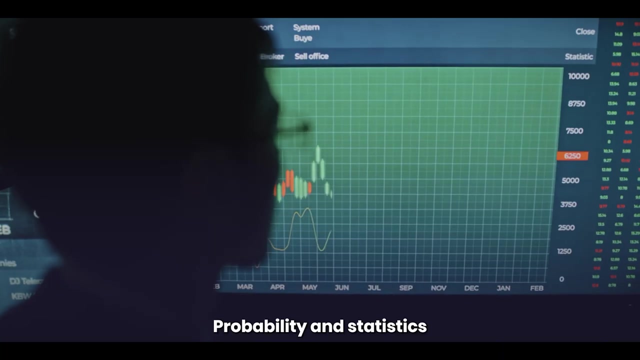 you up for a trial class as soon as possible? Probability and Statistics. Probability and statistics are essential branches of mathematics that deal with uncertainty and variability. Let's take a look at how they can be applied in the real world. Probability and statistics are used in many fields, including economics. 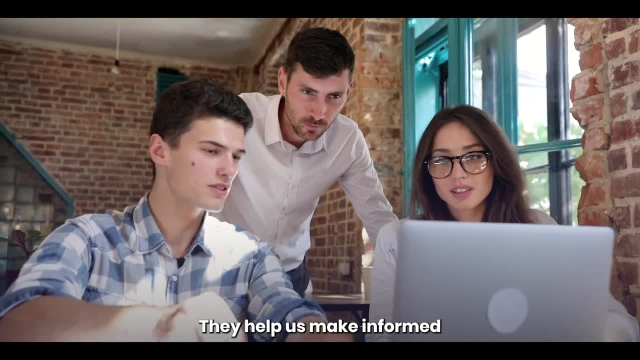 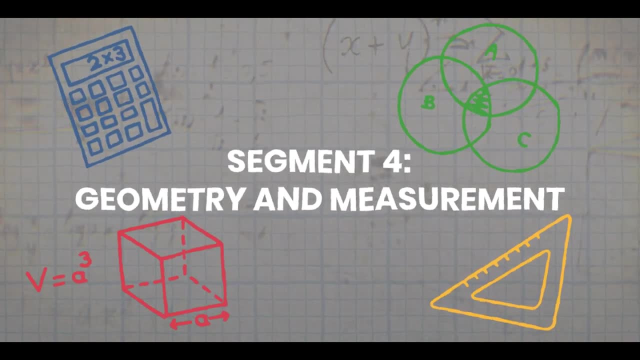 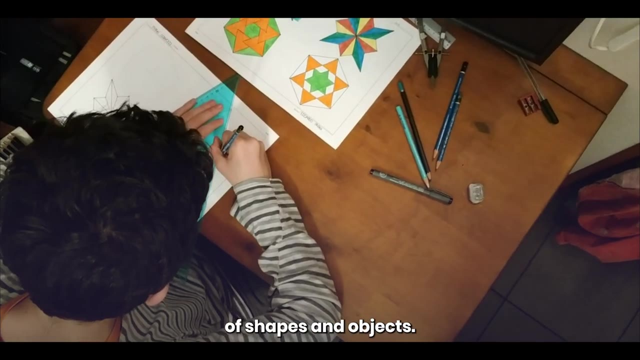 medicine and the social sciences. They help us make informed decisions based on data and reduce the risk of making mistakes. Geometry and measurement. Geometry and measurement are fundamental areas of mathematics that deal with the properties and relationships of shapes and objects. Let's see how they can be applied. 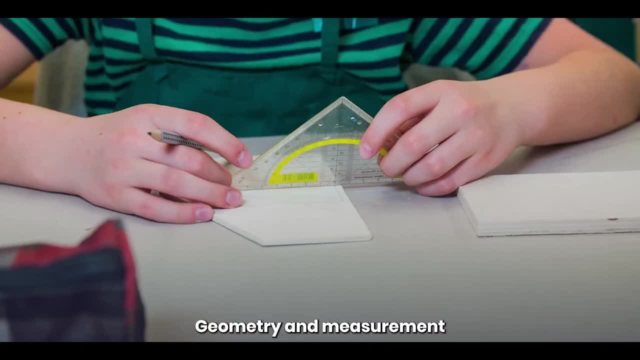 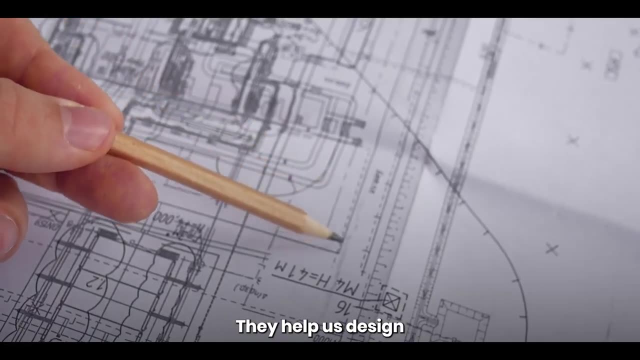 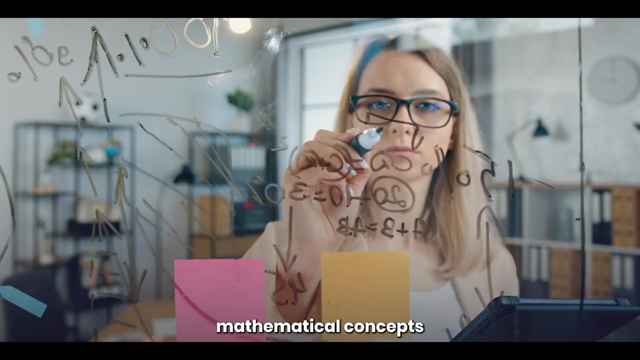 in construction and engineering. Geometry and measurement are essential in many fields, including architecture, engineering and manufacturing. They help us design and construct structures that are safe, efficient and functional. In this video, we've explored some exciting mathematical concepts and demonstrated how they can be applied in 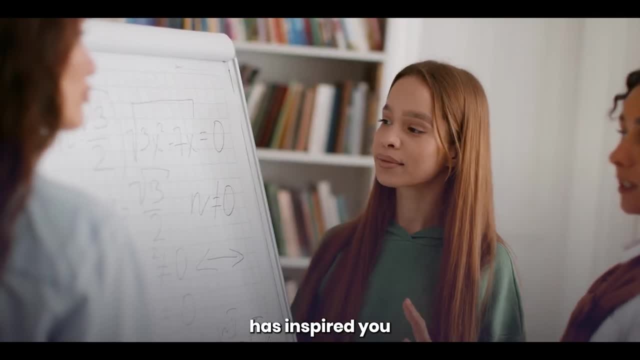 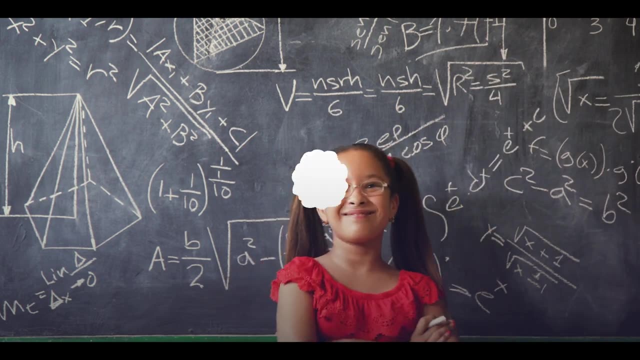 real-world scenarios. We hope this project has inspired you to appreciate the beauty and usefulness of mathematics and to continue exploring its endless possibilities. Thanks for watching and don't forget to like and subscribe.